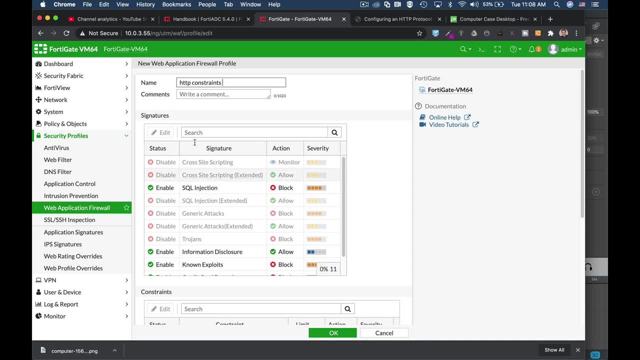 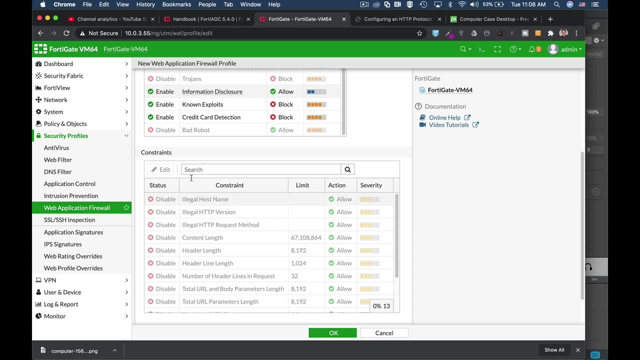 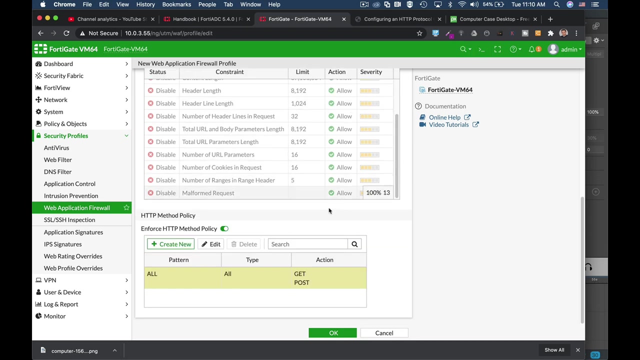 just name it HTTP Constraints, and there you will see the different signatures for known vulnerabilities such as SQL injection, cross-site scripting, credit card detection and so on, And here you will have the constraints which we will configure immediately using our command line. The other thing to note is the HTTP method policy, which 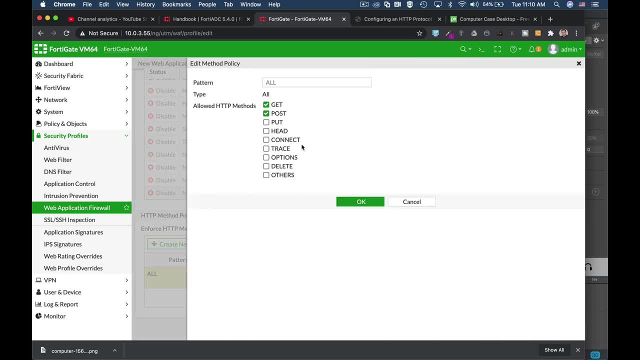 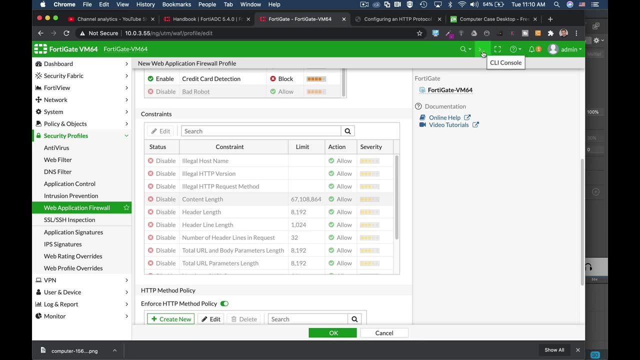 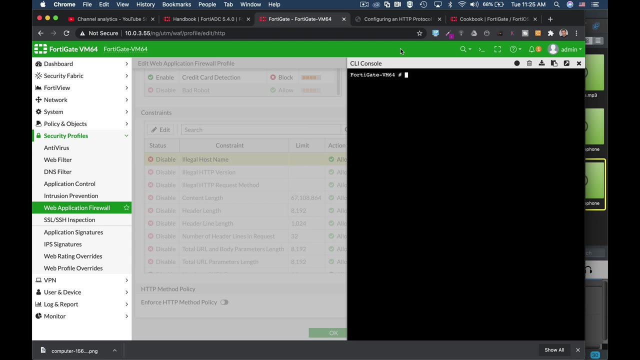 will be matched in the HTTP request, But we will look at the HTTP constraints for now. So let's open our CLI. We're using HTTP constraints to examine web traffic Now. if we find different patterns or inconsistency or something is not in the standard, then it may indicate that there's an attack on our web. 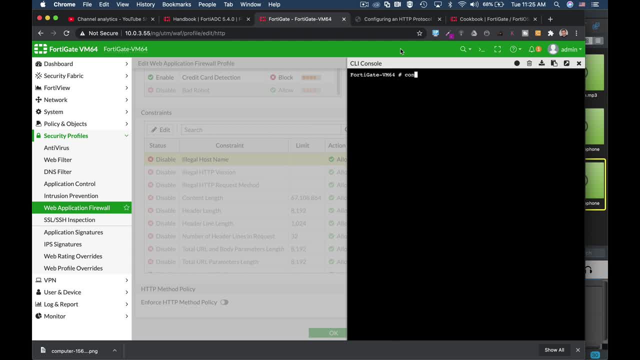 servers. So we configure it using the config WEF profile. Now let's edit my profile, which I named HTTP, and now I will use the show full config to see the constraints. So we can, as you will see, we can configure signatures, we can configure the HTTP methods and we can. 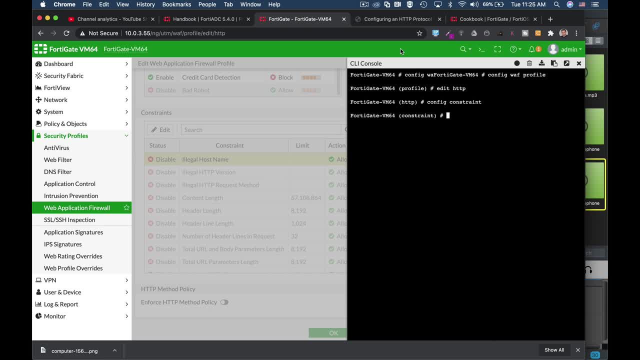 configure the constraints, which we will do right now. Now we'll use the show full config so you can see the different constraints. We have content length, we have header length, that is, the HTTP header length, and so on. But what we will do right now is to configure the constraints, So we can configure the. 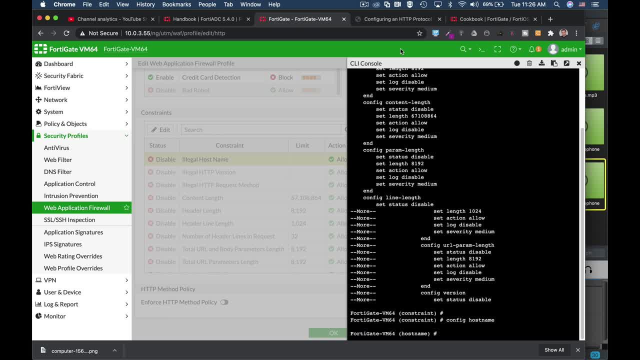 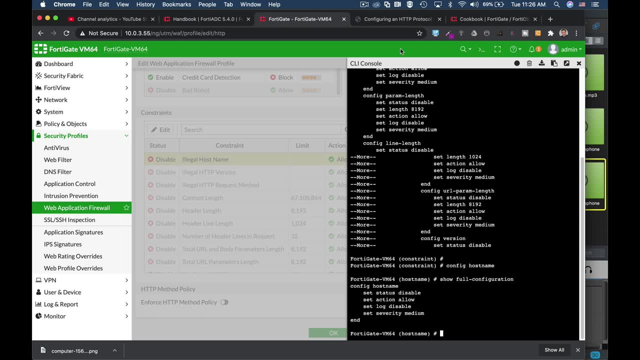 hostname and if we'll use the show full config. by the way, when we configure the hostname, we actually tell a FortiGate to look for illegal hostname. Each hostname has to have its description, its name, in ASCII printed characters. So when we use the bigger sign or lesser sign, then we are actually